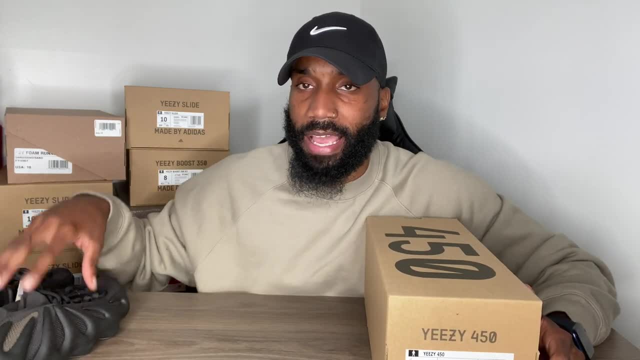 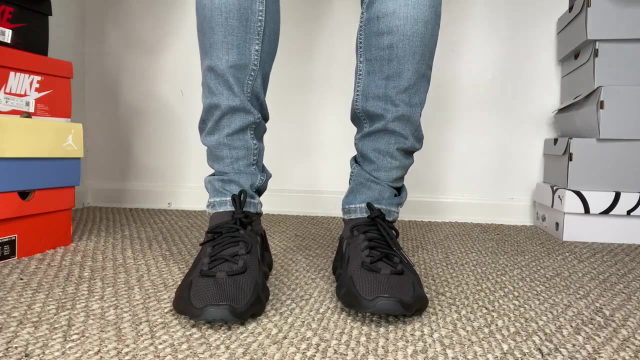 a 9.5 in. Even in Yeezys I would either get a 9.5 or a 10.. I know on the slides I told you guys I got a 10.. You might have to go up to an 11., But on these I got them in a 9.5 and they fit amazing. 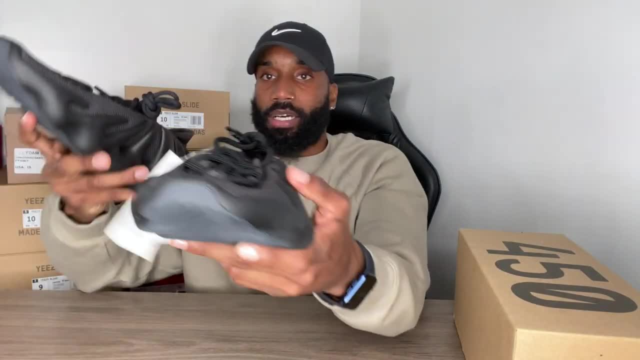 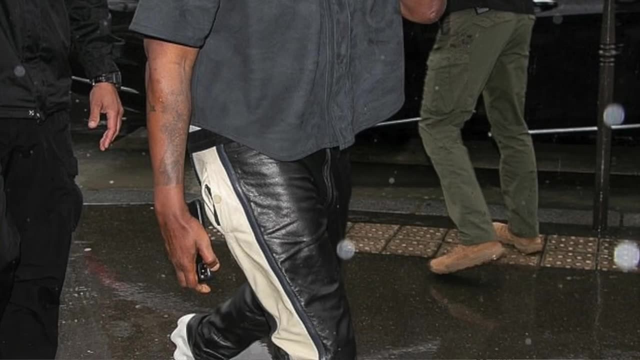 But yeah, let's get right into the shoe. man First looks at it. It's really sexy man. We've seen a picture of Kanye in the white ones in 2018 for the first time And we were all wondering when. 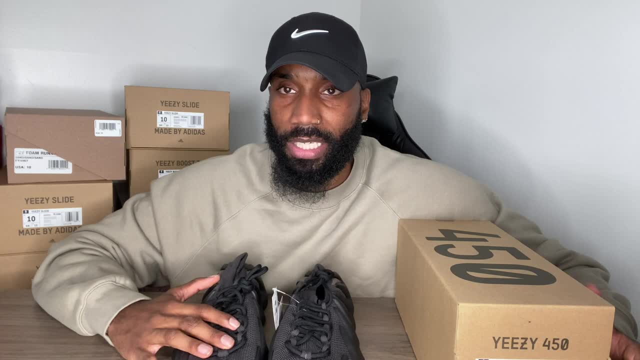 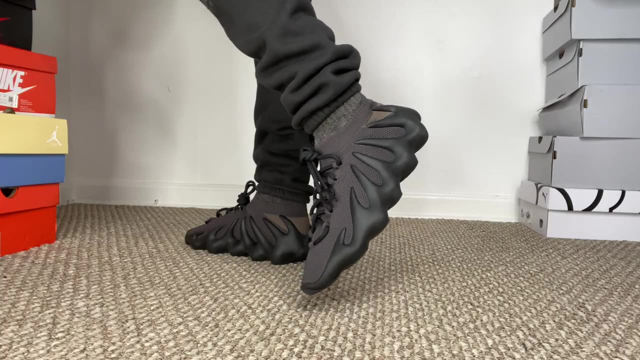 they were going to drop And then they dropped March 6th 2021,, I believe, of this year, And then now, June 25th 2021, we get the dark slate right here And, wow, these are just amazing and sexy. 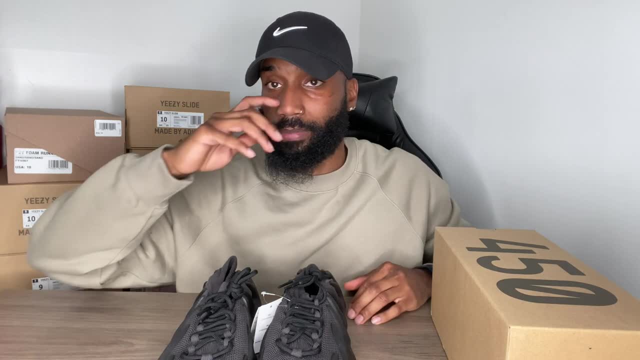 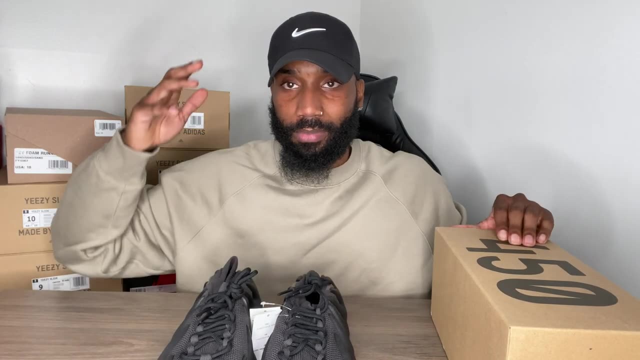 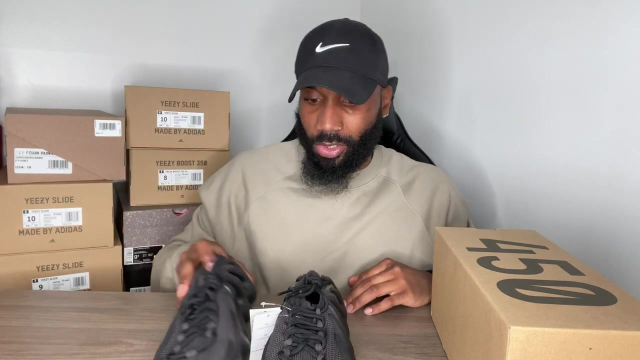 I believe on the Adidas Confirm app. actually, the raffle is still open, So you guys can join that. Don't quote me on that, though, because this video might go up after that, But here we are today, live with the 450 in hand. So yeah, let's get right into it, man. So starting. 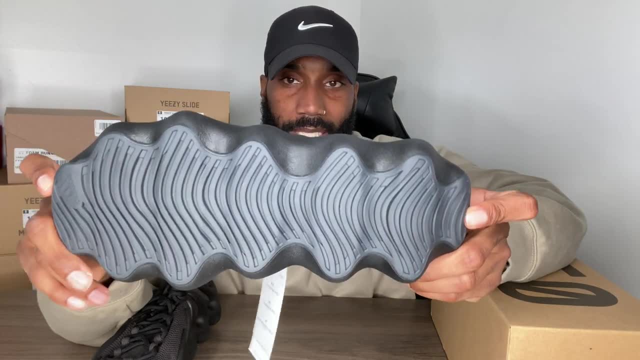 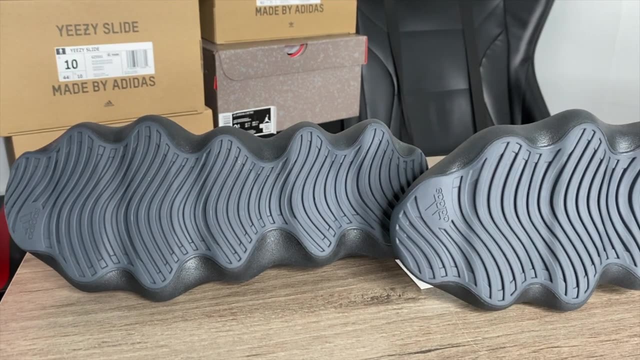 off with the bottom of the shoe it's in an all black. But then when you put it up to like some light or the camera, it kind of looks like a navy on the traction back there. So maybe it's just a light making it look like a navy blue, But then when you take it off the light it looks black. 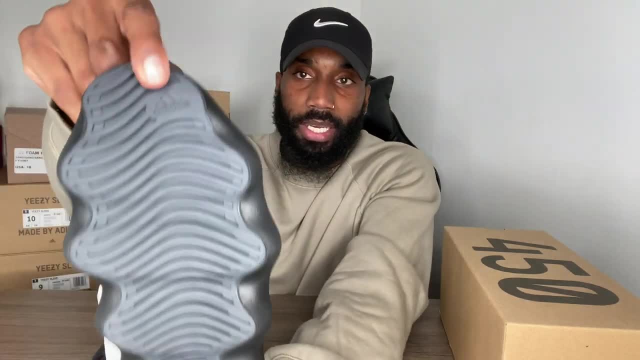 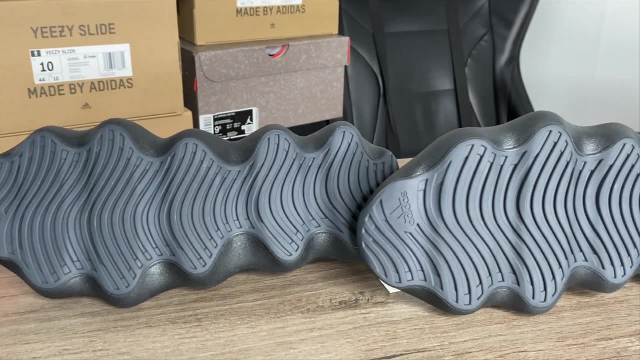 to the eye. The only thing that tells us that it's an Adidas shoe is that it says Adidas right there at the top of the shoe. It doesn't say Yeezy or Adidas anywhere else on the shoe, which is pretty cool. I don't like my clothes to have a lot of branding names on it And if I do, I want it to be. 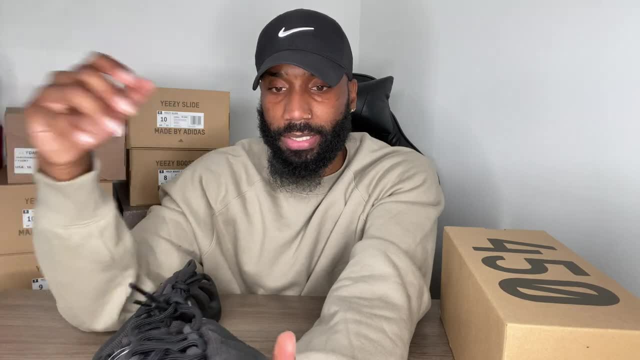 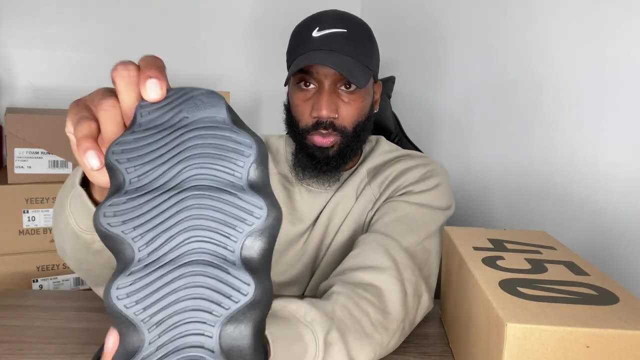 very small, and you'll just have to know what I'm wearing to know what it is. But yeah, also, it just looks like some waves, too, are just going up and down the shoe here, which is pretty dope. If you look at that from the side too, it does look like some waves going up and down the shoe, which is 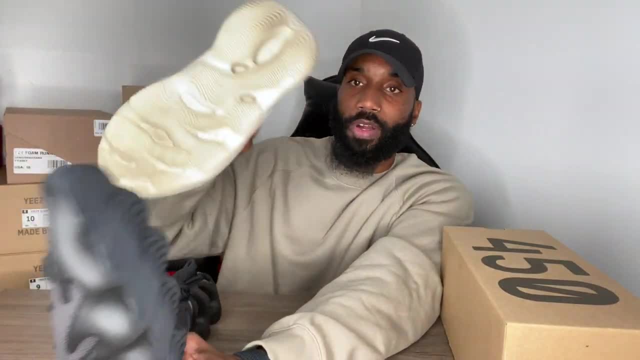 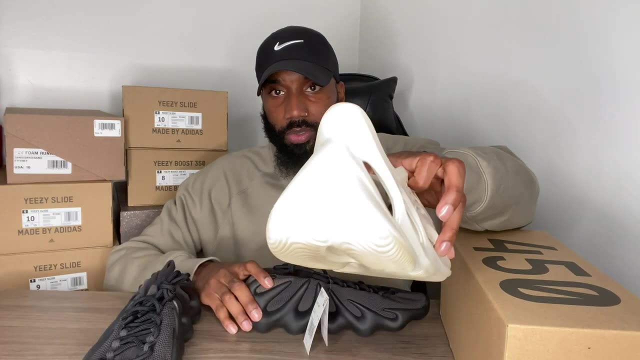 kind of similar to the runner that I have on right now. I have been wearing these like every day since I got them And they also have some similarities with that slope going up at the back. show you that slope thing going up at the back here. Same thing with this one going up here. So 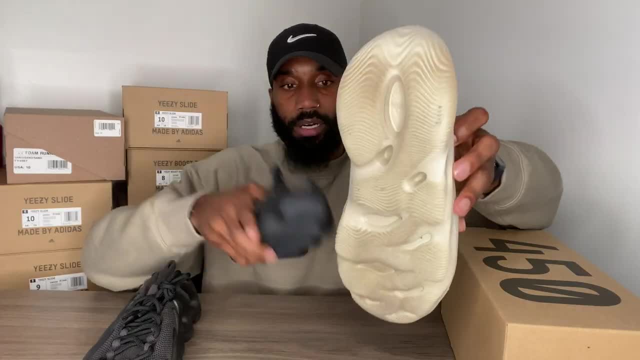 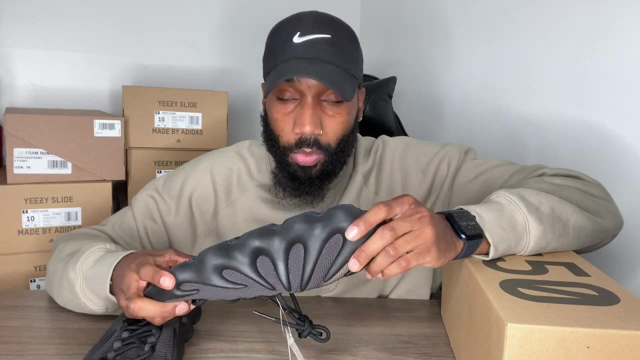 that's some similarities. So show you guys that. But yeah, man, you guys know everything touches the toe. So, man, I'm going to have to give these the wears of my life. But man, these are really fire. just looking at the bottom of it, You just see like that wave pattern going down the shoe. 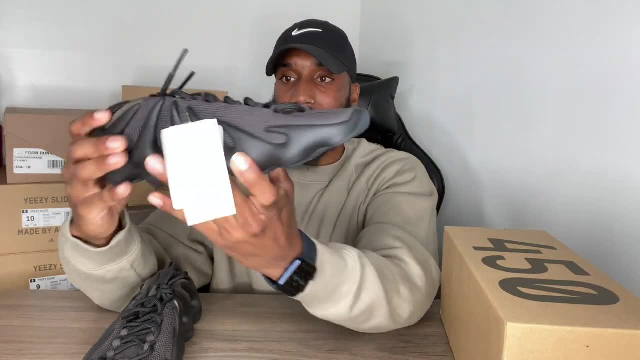 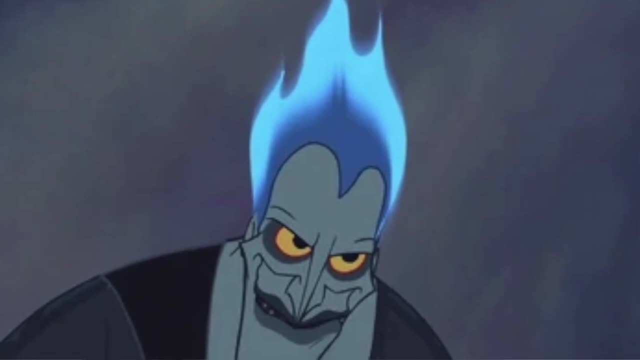 coming up to the midsole of the shoe. In my opinion, looking at it on both sides, like some flames going up The shoe, which is pretty dope in my opinion. I can't wait to see what other colorways come out. 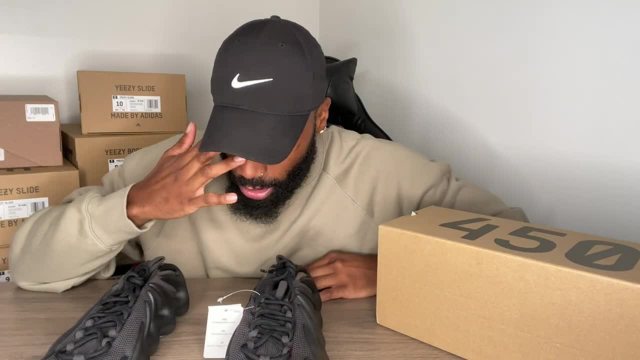 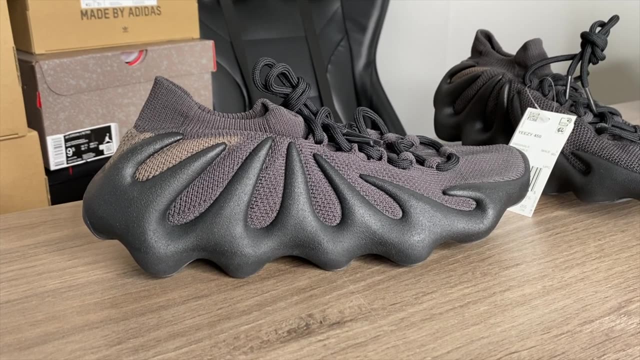 later in the year. Again, these do not come with boost technology. It comes with EVA foam, which we see here on the bottom of this midsole, If you guys look at it, because I mean, this is just a solid color, a solid, futuristic looking shoe, In my opinion. 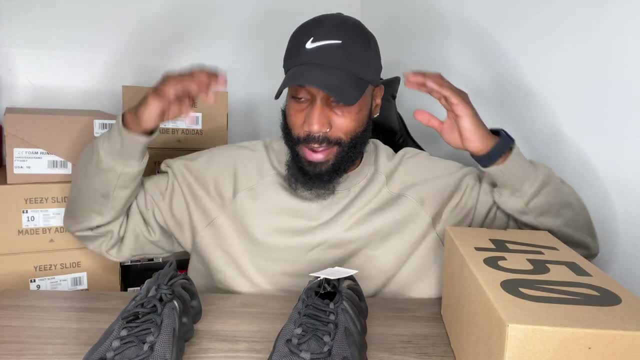 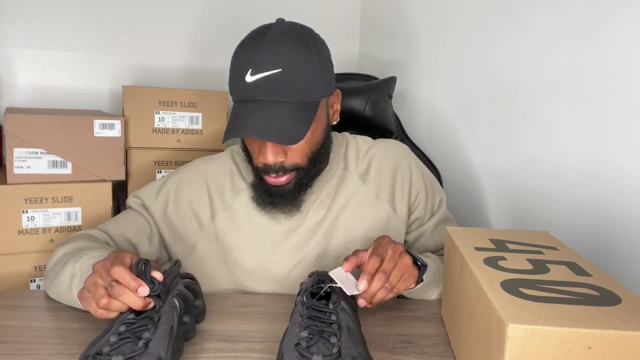 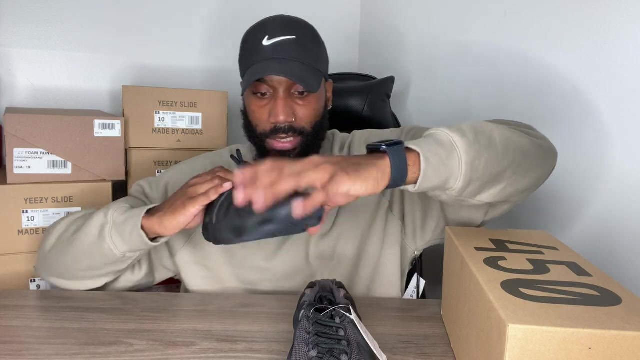 Yeezy is just keeping Nike on their toes and just dropping banger after banger after banger. This month has been another crazy month for Adidas. It's been Yeezy, but now the rest of the shoe is basically like in a prime knit here, So it's just. 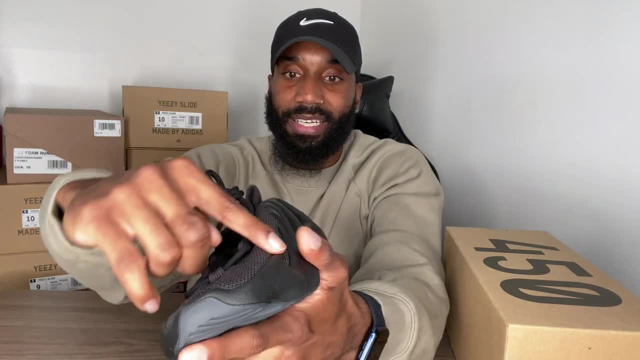 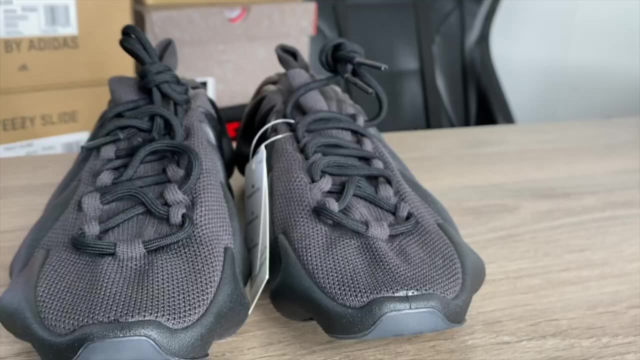 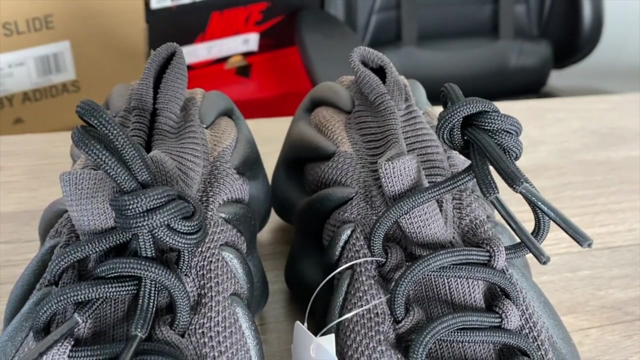 like a. well, the correct term for it is dark slate, So it's in a dark slate prime knit going around the shoe here, all the way around the shoe, even on the eyelids. We have some like shoelace holders here and they like hold the laces in there, which we only get one pair of. 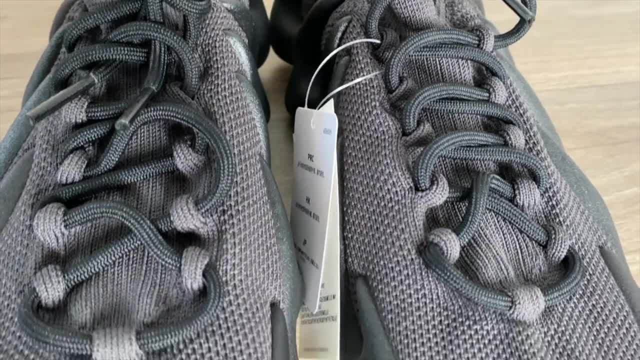 We only get one pair of black laces and a rope style lace too. We only get one pair of black laces. We only get one pair of rope style laces on this, on these. but yeah, we get some eyelids and they. 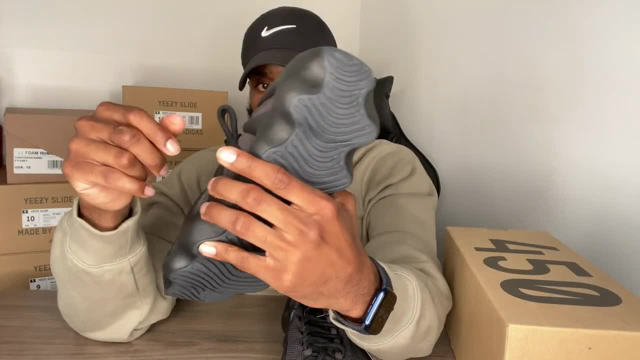 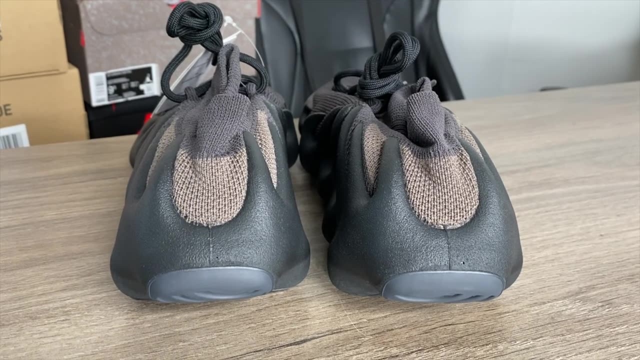 just hold hold in the sock here which have some give. you know what I mean. So on the back of the shoe here it's in like a brownish color- earth brown, I don't know, but it doesn't say anything. 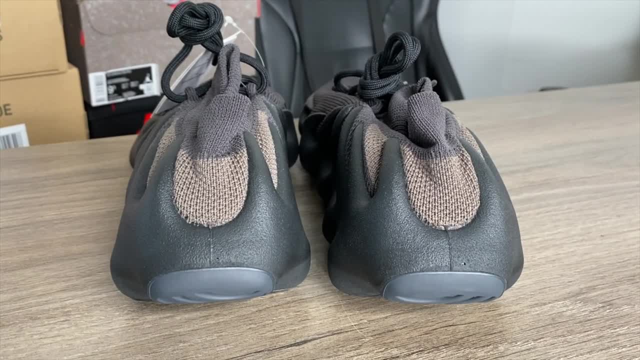 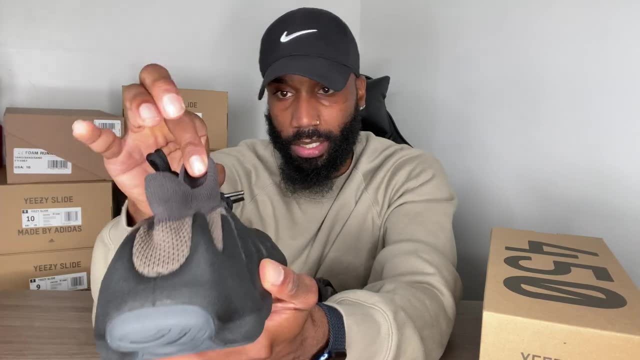 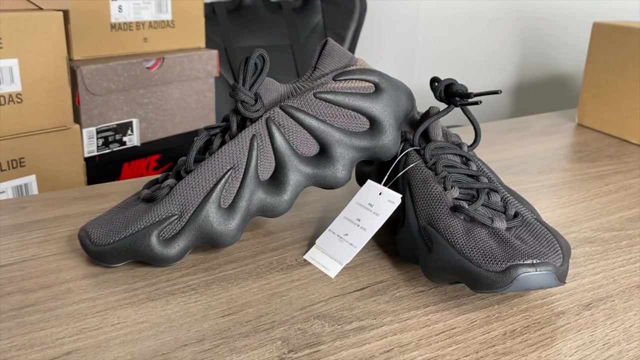 about that on the box. but yeah, it doesn't say anything about that on the box, but it's like a brownish back there. And then at the top it goes back to that dark slate color, Which is pretty dope, And it's just like a sock. Basically, the whole shoe is basically like a sock. 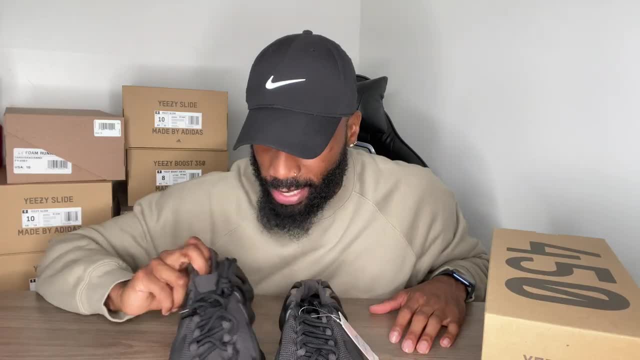 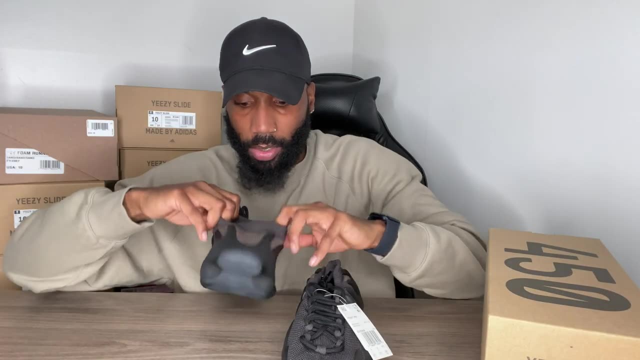 and molds to your foot. If you have three fifties, it's basically like that, but just a different midsole because it has like that same sock, but it fits different. Now again, I did go, I did get a nine and a half in these and they fit amazing. They don't fit as snug as a three 50. 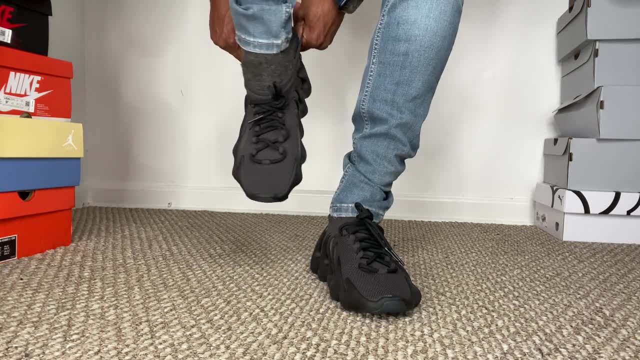 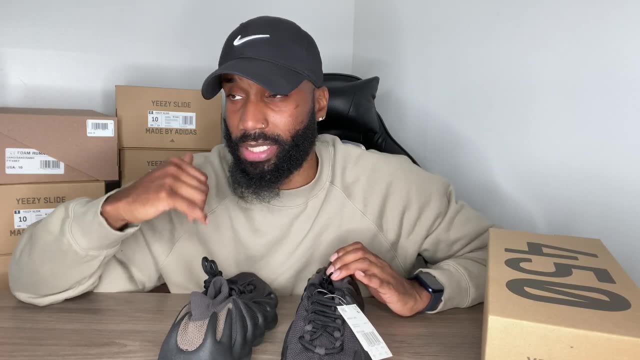 would Um. so in my opinion, you only have to go half a size up. I normally wear nine, but I get nine and a half in everything Slides I had. I got them in a 10 and I believe you need an 11, but that's just my opinion. 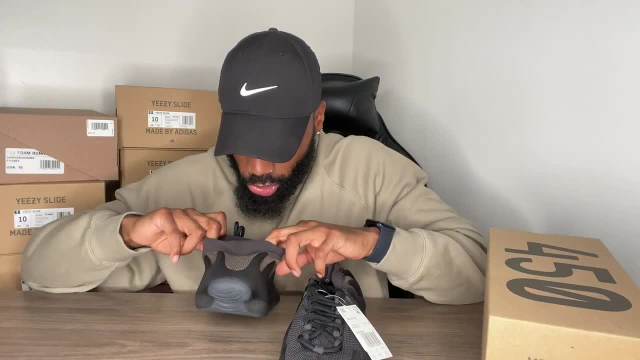 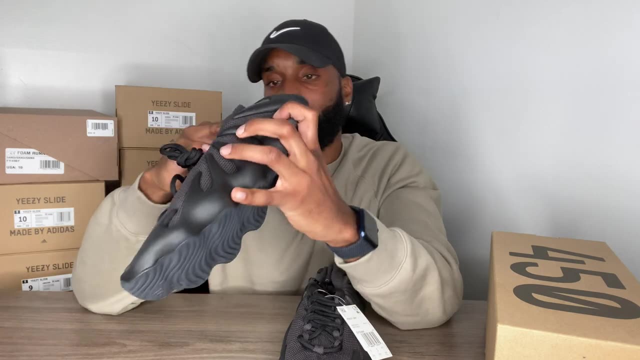 So I did go half a size up. um, on the inside of the shoe here it's all blacked out and it says Yeezy ortho light in there. Um, let me take out the sole for you guys, And so. 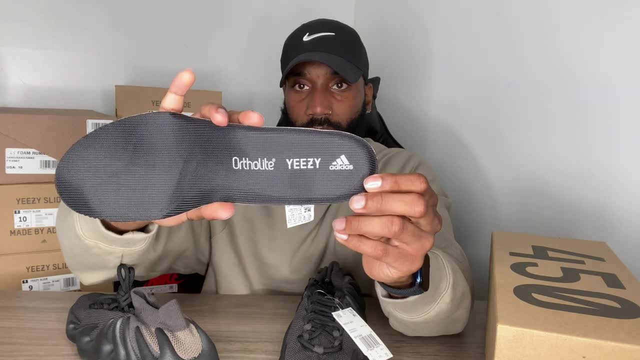 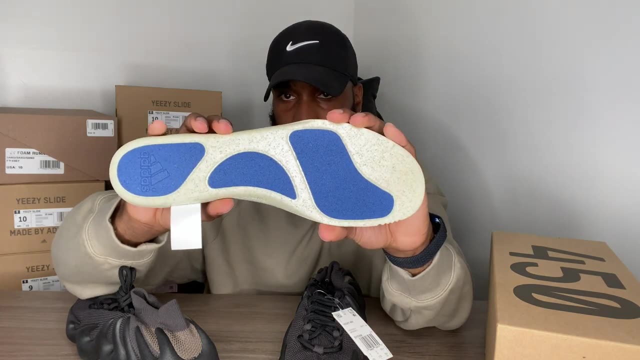 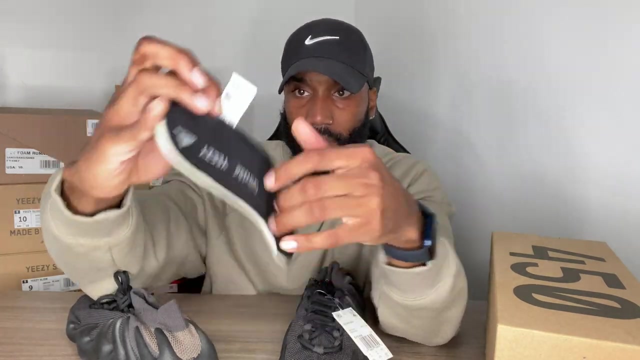 and the insole is in black and it says Yeezy ortho light. Then it has that Adidas logo right there on the bottom. It's blue and gray. Okay, Now on a tag here. we get a tag here and it just says the sizing and everything. Also, it says: 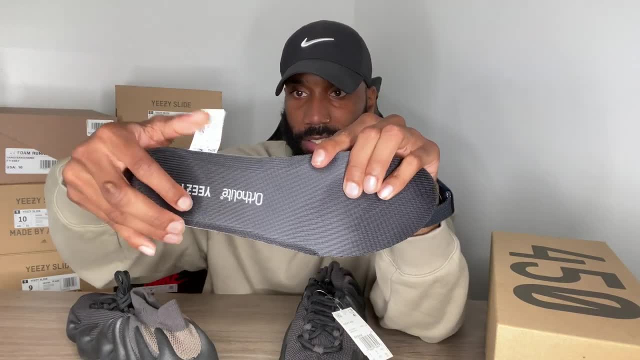 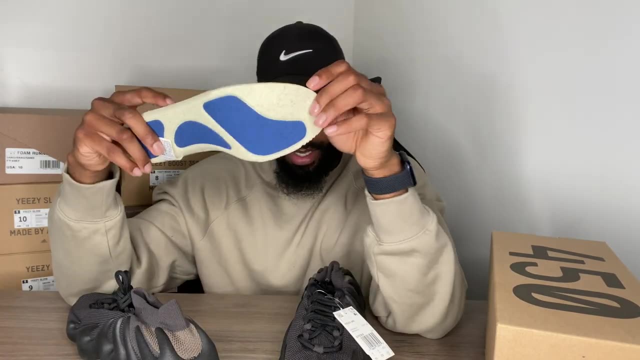 flip under. So if you don't want this showing on the inside of the shoe, you can flip that under just like this, and it won't sort on the side of the shoe, which is pretty dope. I didn't know that until just now, Um, but yeah man, all around a really dope shoe. I believe retail on these was. 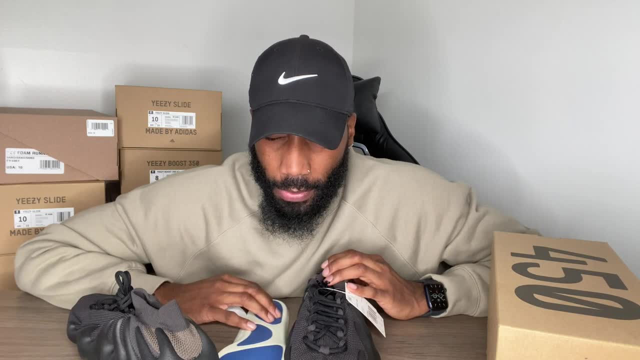 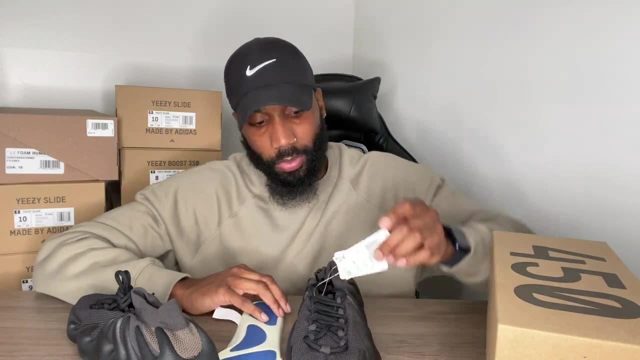 200 and resale is going for like 400 right now. So I believe this shoe is going to go up Like again. I can't wait for other colorways To come out. Um, we do get some two tags on here. Always look them up into the light and then see if. 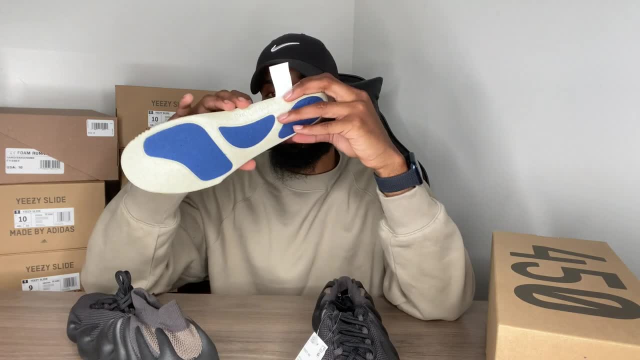 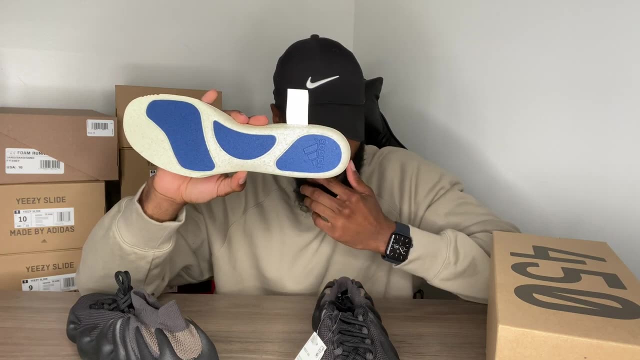 I can see through it a little bit, Then they'll find out real. Also, you might want to check your pairs. I seen somebody with a pair and he had like yellow on the bottom, but I don't know. I don't know, man, I just know mine come with blue, So make sure yours come with blue. I'm